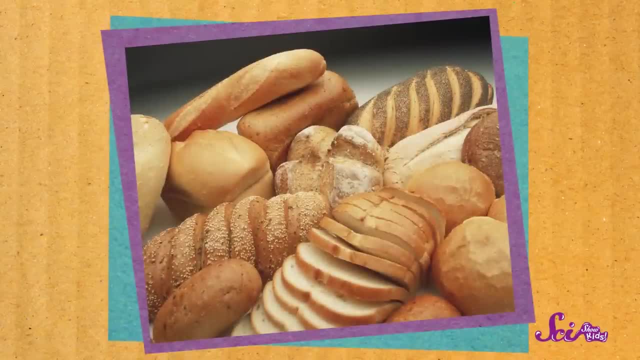 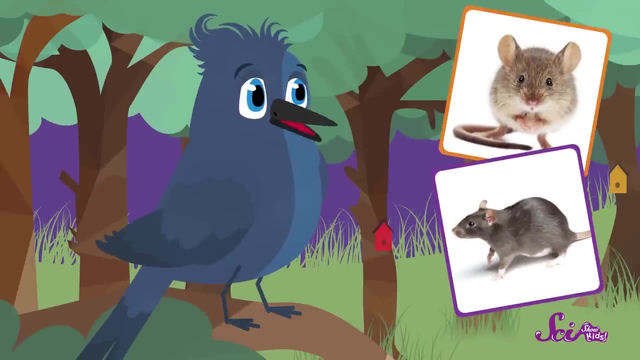 Thank you in advance. Another food you should avoid is bread. I mean I'll eat it, but it doesn't really give me the nutrients that I need. Plus, it can attract mice and rats, And as good as I am about sharing, I do like to have my food all to myself. 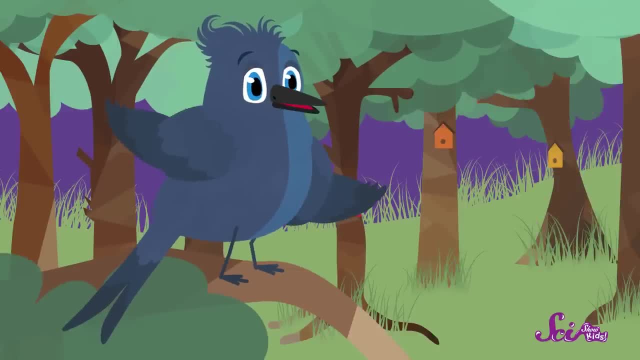 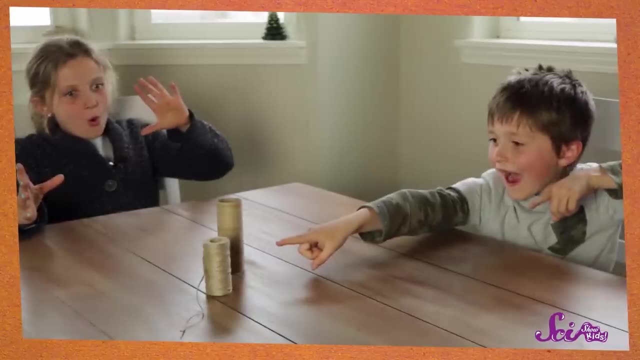 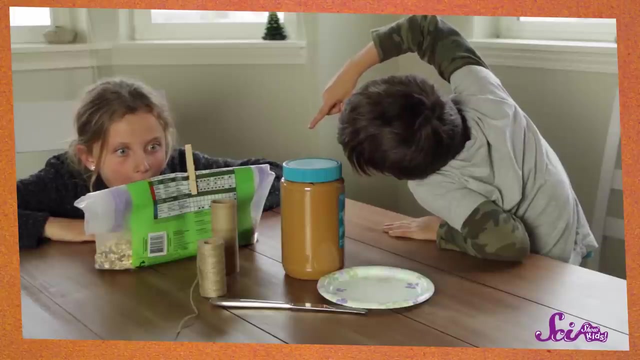 Now that we got our food basics down, let's make some bird feeders. This one is really fun and easy to make. All you'll need is a toilet paper roll- Eh, I said toilet paper- And also some string, some peanut butter, a butter knife or a spoon, a plate and some bird food. 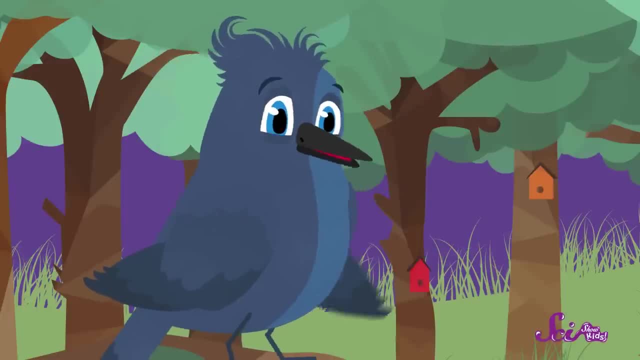 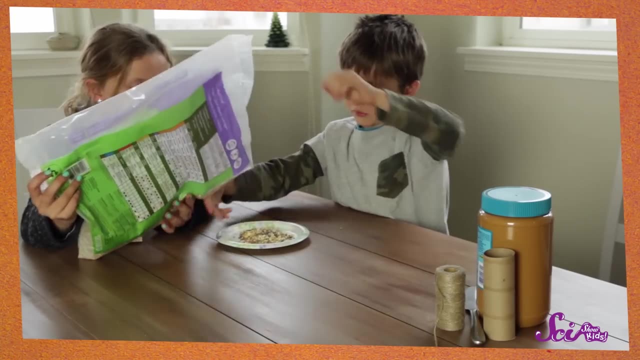 And may I suggest my personal favorite sunflower seeds? Yum, yum, yum. Now this might get messy, so make sure you're in a place where it's okay to make a mess. First, set out your plate and pour some bird seed on it. 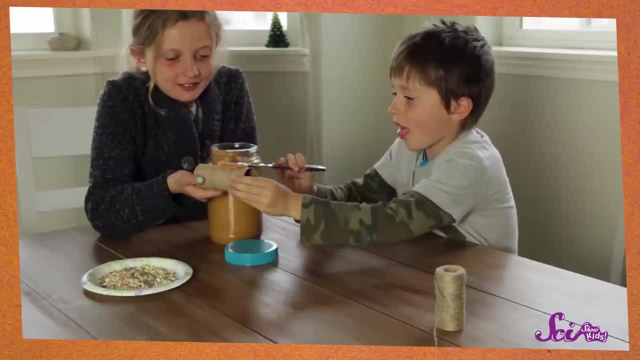 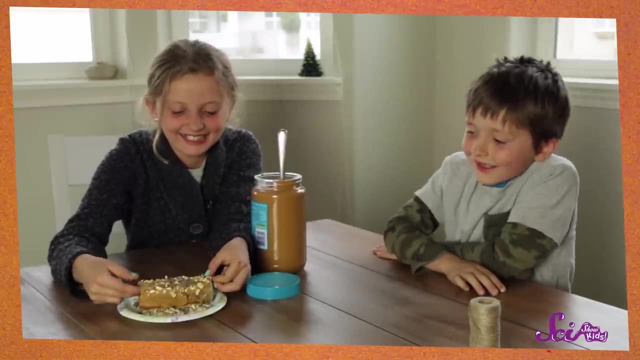 Set this aside for now. you'll use it later. Take some peanut butter and spread it all over your toilet paper roll. Yeah, you're on the right track. Next, Roll your toilet paper roll across the bird seed until it's well covered. 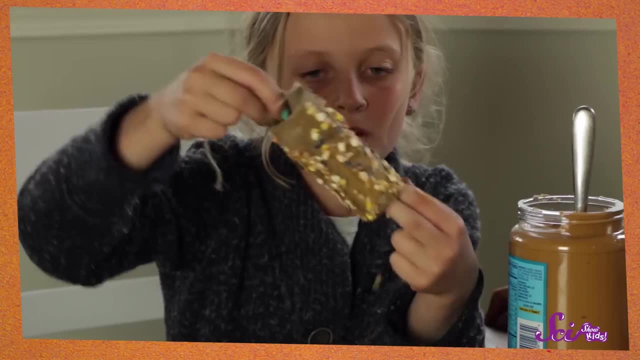 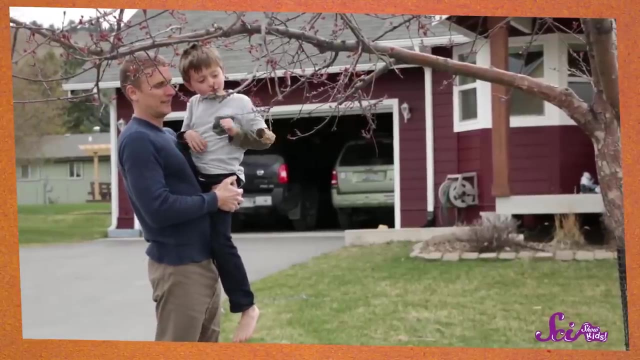 You're almost there And I'm starting to drool. All you have to do now is pull your string through the middle of the roll, Then just tie your bird feeder to a tree. That'll be a great place for me to take a quick snack break later. 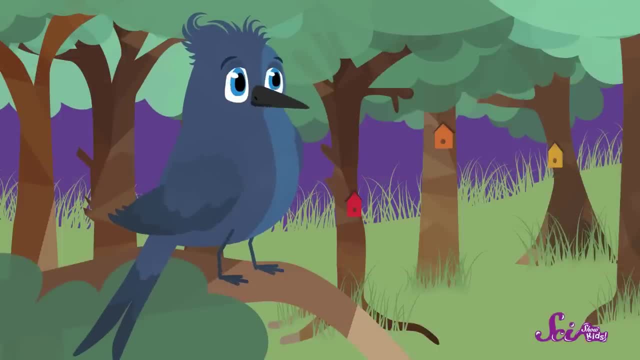 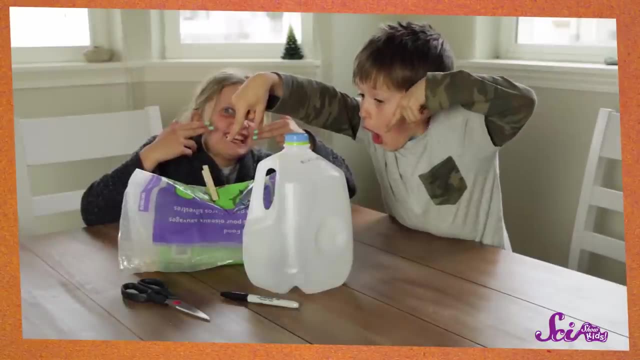 This next bird feeder is really fun because you can keep filling it up over and over. You'll need an empty plastic jug, a marker, bird seed and scissors For this feeder. you should ask for help from a grownup First. draw a circle on one side of the jug. 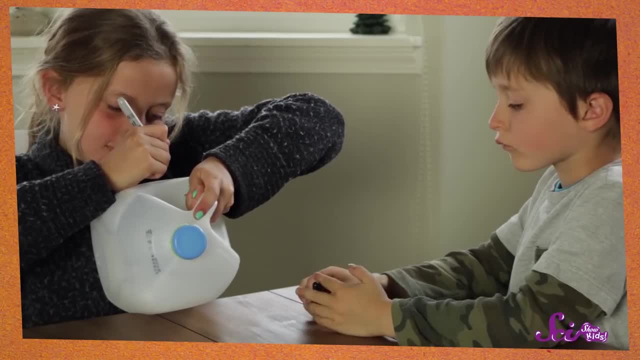 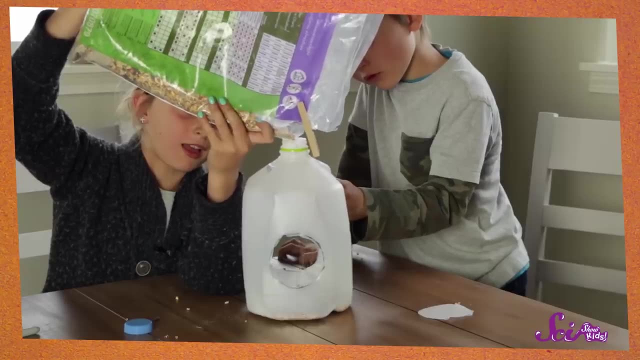 Where you want your birdie friends to get their food. On the opposite side, draw another circle. Next, ask for help from a grownup and cut the circles out. That looks great. Now you can fill your feeder with bird food. 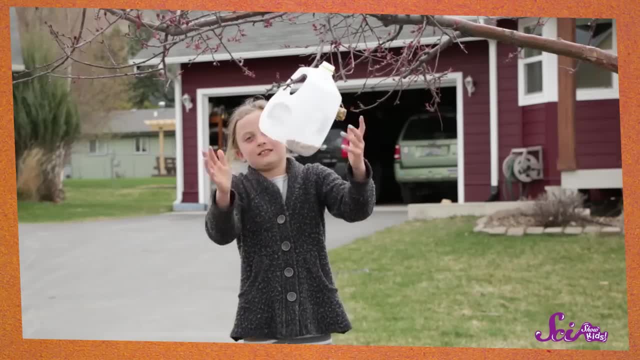 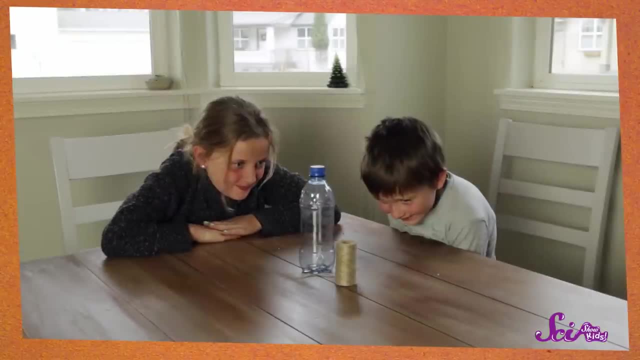 And finally, you can hang your bird feeder on a branch using the jug's handle, No string needed. Okay, I have one more fun bird feeder to show you. that's really easy to make. All you'll need is an empty plastic bottle, some string, scissors, bird seed and a wooden spoon. 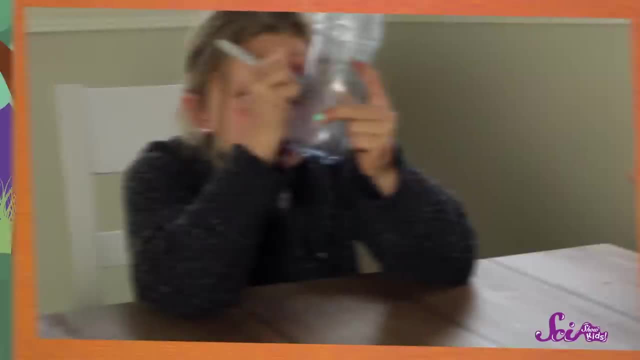 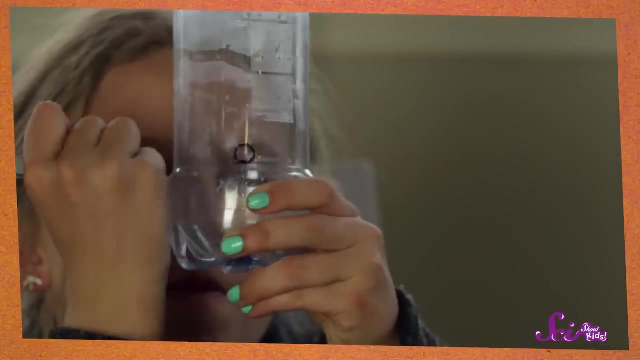 And if you have an extra pencil lying around, that'll work too. First mark a spot on the bottle, near the bottle, About the width of your wooden spoon or pencil. Now flip your bottle over and mark a spot opposite the one you just made.